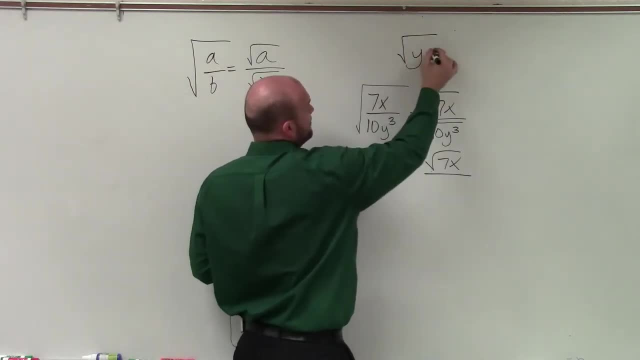 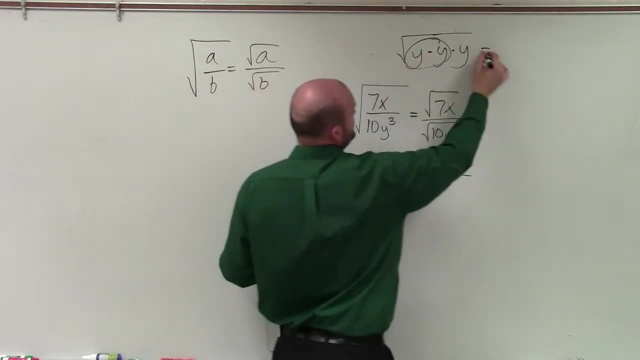 I can take the square root of y squared, because I can break that up into y times, y times y, where I can now group a pair of y's, And therefore I can take that out, which is just going to be left with y times. 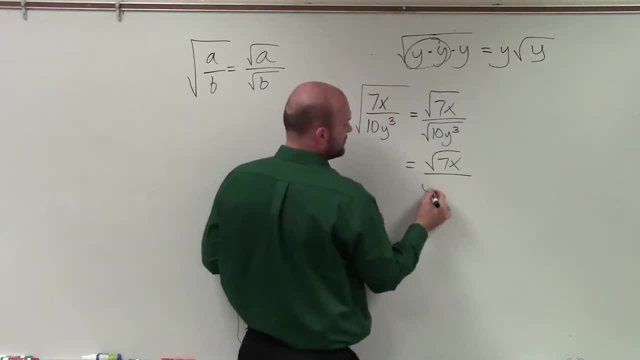 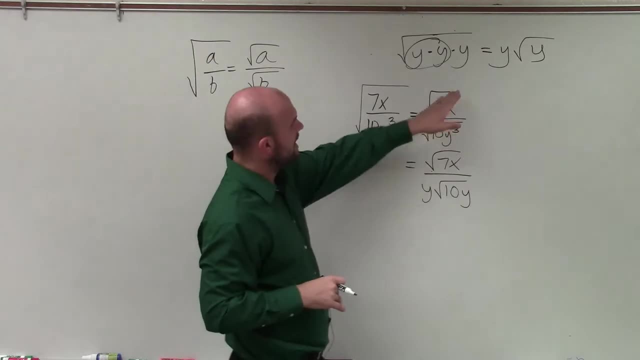 the square root of y, 10 will still be under there. So I'm left with y times, the square root of 10y. All right, So now I simplified: the y cubed into y times square root of y and the 10 had to be down there. 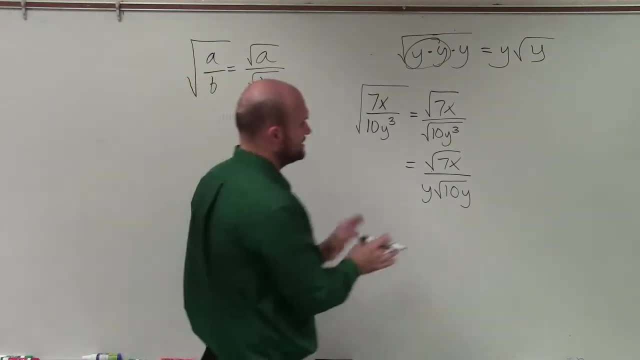 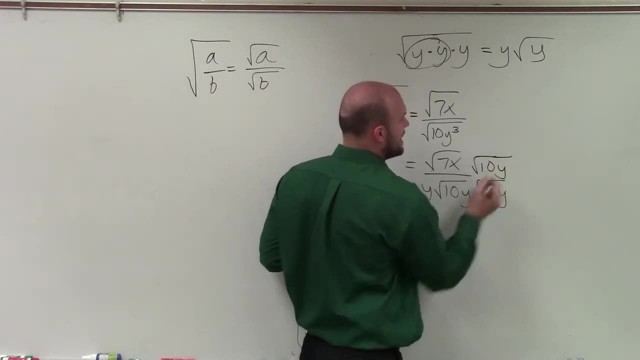 Now I need to get rid of the square root of 10y. So to do that I need to rationalize the denominator by multiplying by the square root of 10y on the top and the bottom, And as long as I multiply on the top. 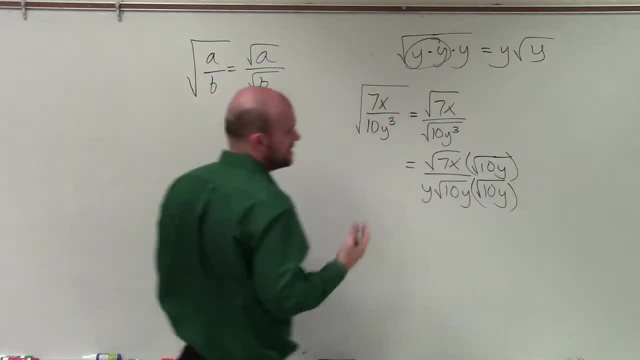 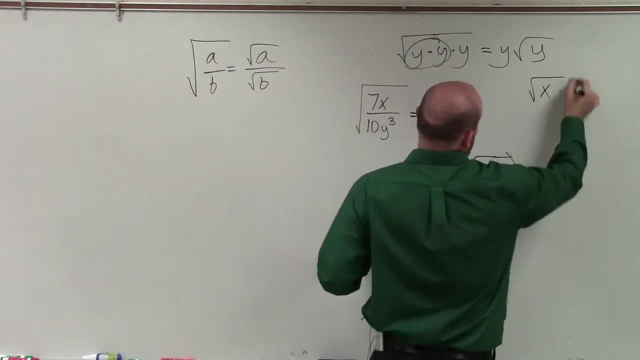 and the bottom I'm going to produce an equivalent fraction, So I'm not going to be changing the answer. But what's important about this is the square root of any number multiplied by itself. for instance, just the square root of x times the square root of x. 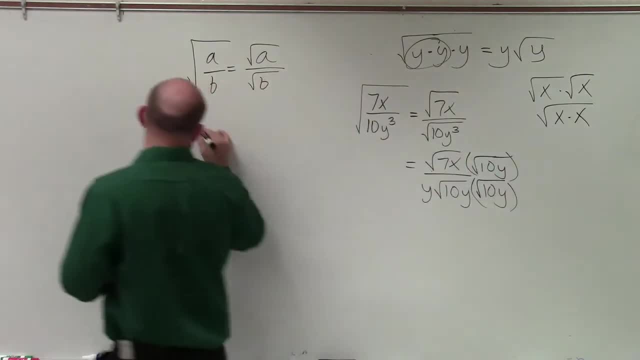 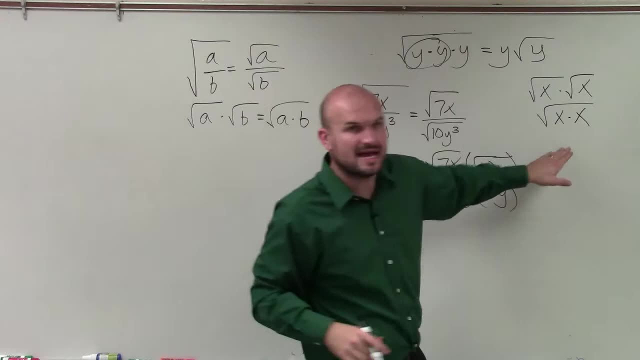 equals the square root of x times x, which is the same thing that we have here a times the square root of b is equal to the square root of a times b. Well, since these numbers are the same, I can pair them up and take the square root. 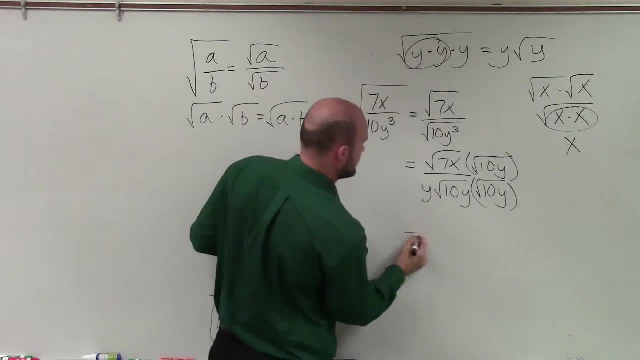 of a pair of numbers which is just going to equal x. So therefore, here, My denominator is just going to be the square root is just going to be 10y. Then, over here, I can multiply my two terms inside my two terms under each radical. 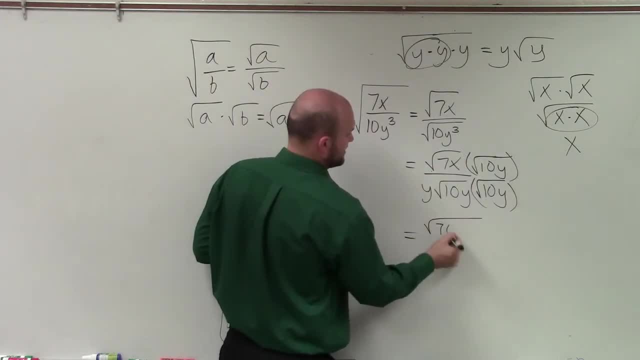 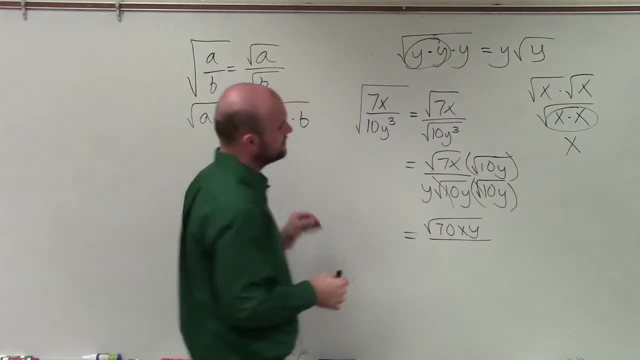 So therefore, I have 7 times 10,, which is going to be 70.. x times y is just going to be xy, And then my denominator, my two square roots I'm going to cancel out And I'm just left with. 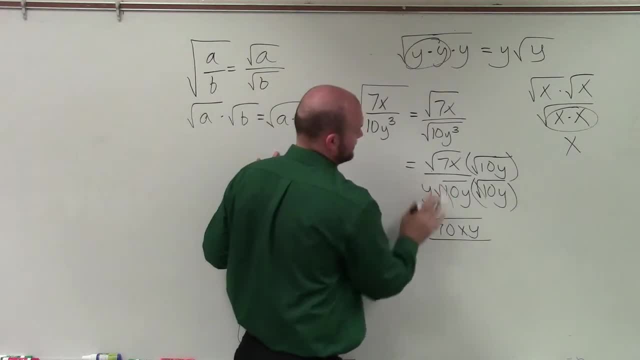 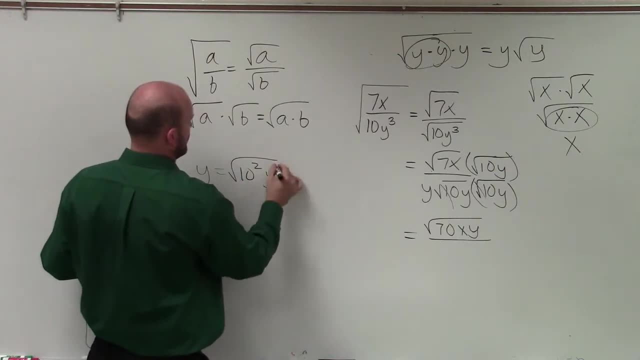 Oh, This is going to be xy. Oh, This is going to be xy. No, Geez, don't mind me. So what this becomes is: y equals the square root of 10 squared y squared, which is just equal to 10y. 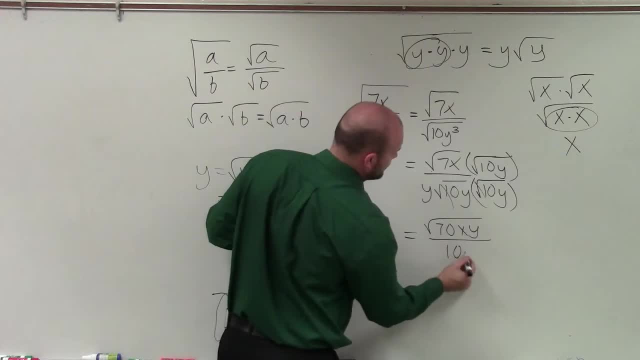 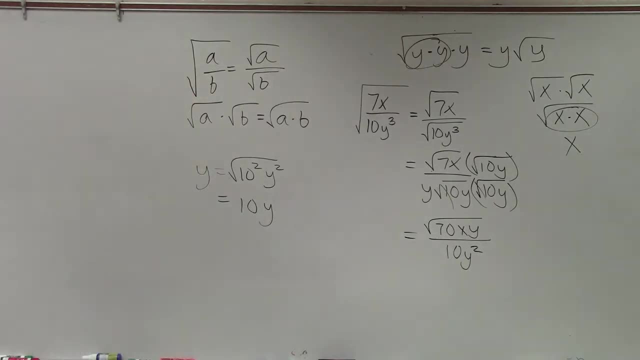 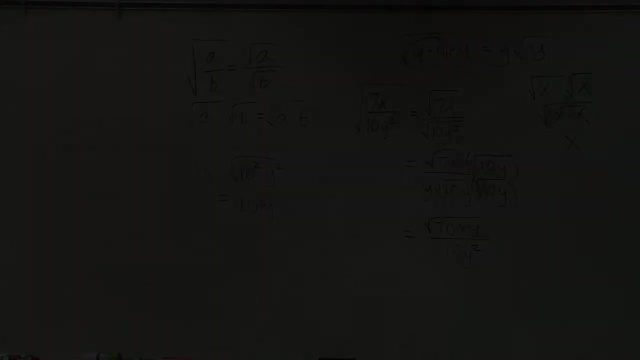 So, therefore, 10y times y is going to be 10y squared. So there you go, ladies and gentlemen. That is how you simplify your radical expression. Thanks, Thank you.